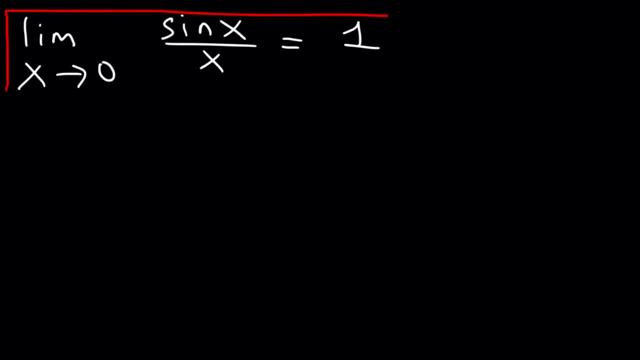 So now let's confirm it. A nice simple technique to evaluate any limit, if you have access to a calculator, is to plug in a number that's very close to what x is approaching to. In this case it's approaching 0, so let's try 0.1.. 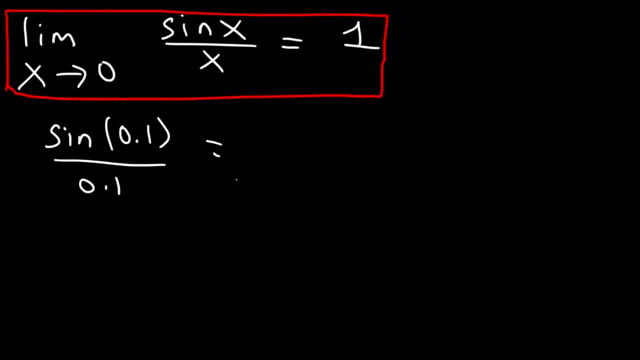 Make sure your calculator is in rating mode. by the way, Sine of 0.1 divided by 0.1. That's equal to 0.998, which is very close to 1.. Now let's try 0.01.. 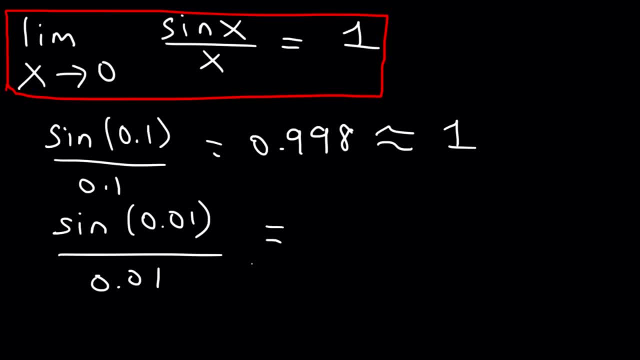 Let's see what's going to happen. So this is going to be 0.99998, which is even closer to 1.. So we know that this equation holds true. Now there's another formula that you need to know. It's the limit as x approaches 0, 1 minus cosine x divided by x. 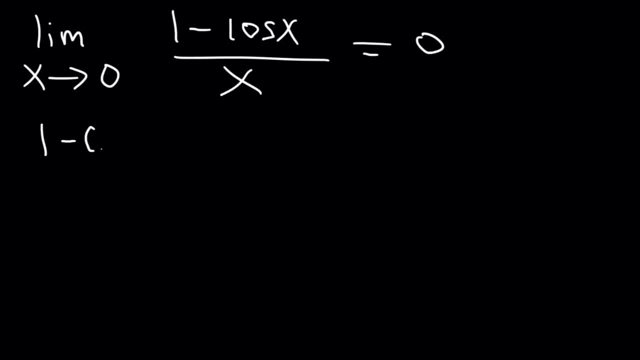 This is equal to 0.. So to confirm it, let's plug in 0.1.. Let's see what number we're going to get if we do this. So this is going to give you 0.05, approximately It rounds to 0.05.. 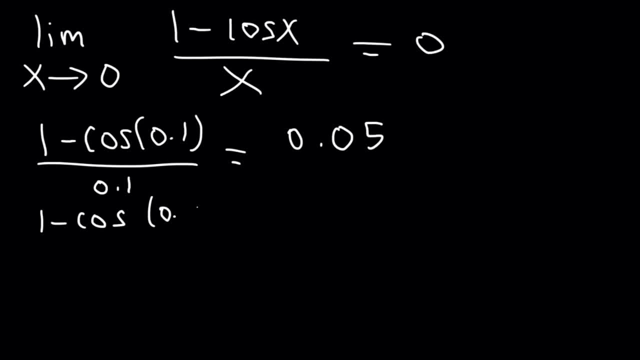 Now let's try an even smaller number. Let's try 0.01.. So this will give you 0.005.. Notice that these two numbers are not the same. They look similar, but this number is 10 times smaller. 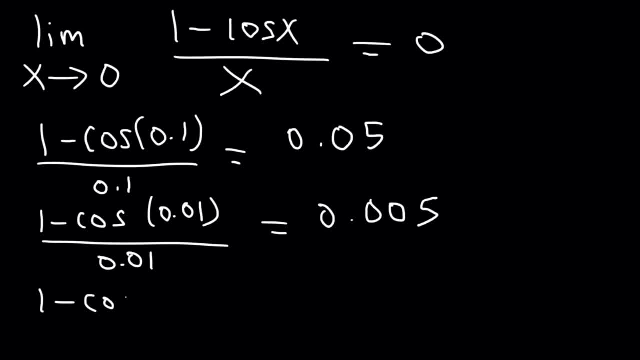 It's getting closer and closer to 0.. Now, just to confirm it, let's try an even smaller number: 0.001.. So this will be 0.0005.. So, as we can see, as x gets closer and closer to 0, 0.005.. 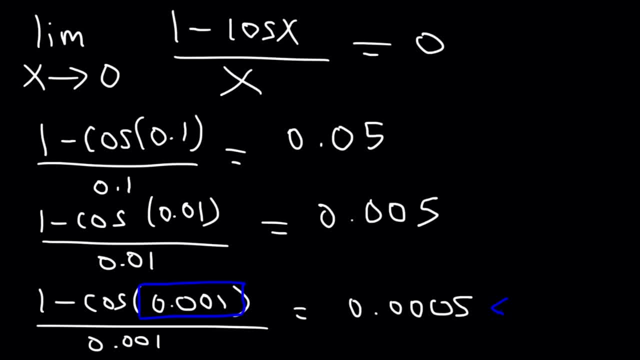 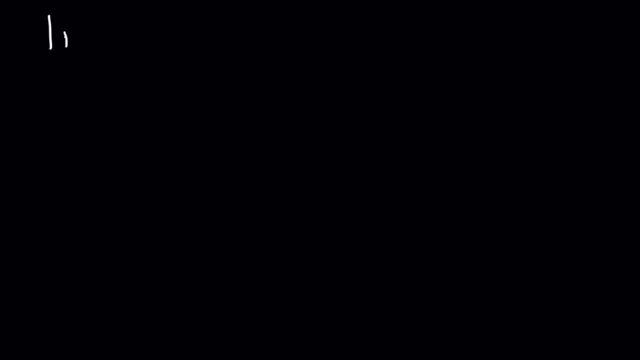 0.005.. 0.005.. So y approaches 0 as well. So this equation holds true. Now let's work on this problem. What is the limit, as x approaches 0, of sine 5x divided by x? 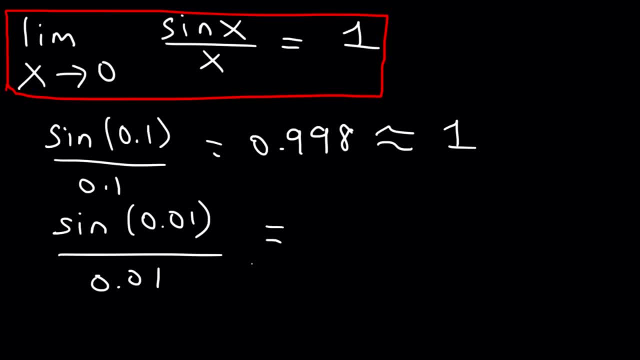 Let's see what's going to happen. So this is going to be 0.99998, which is even closer to 1.. So we know that this equation holds true. Now there's another formula that you need to know. It's the limit as x approaches 0, 1 minus cosine x divided by x. 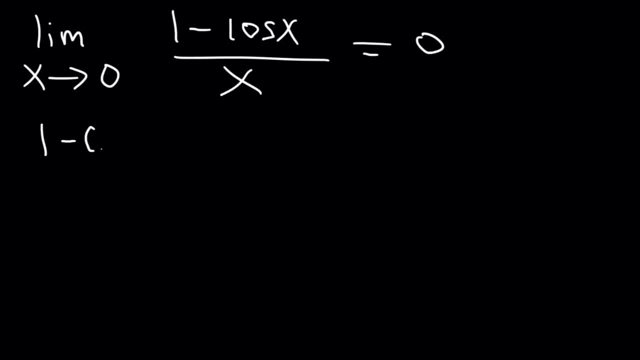 This is equal to 0.. So to confirm it, let's plug in 0.1.. Let's see what number we're going to get if we do this. So this is going to give you 0.05, approximately It rounds to 0.05.. 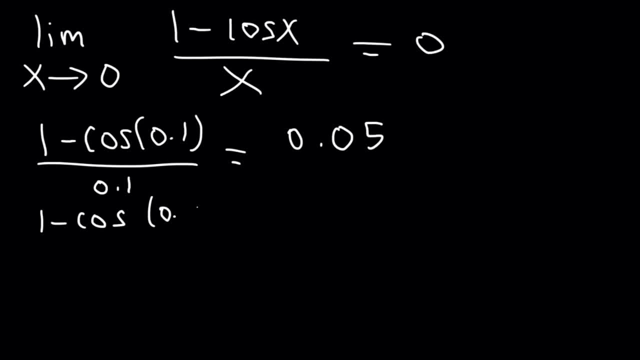 Now let's try an even smaller number. Let's try 0.01.. So this will give you 0.005.. Notice that these two numbers are not the same. They look similar, but this number is 10 times smaller. 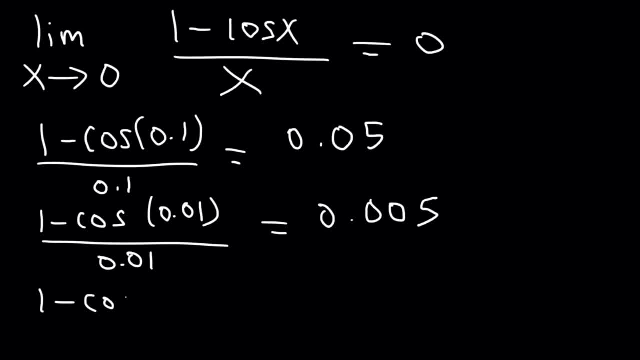 It's getting closer and closer to 0.. Now, just to confirm it, let's try an even smaller number: 0.001.. So this will be 0.0005.. So, as we can see, as x gets closer and closer to 0, 0.005.. 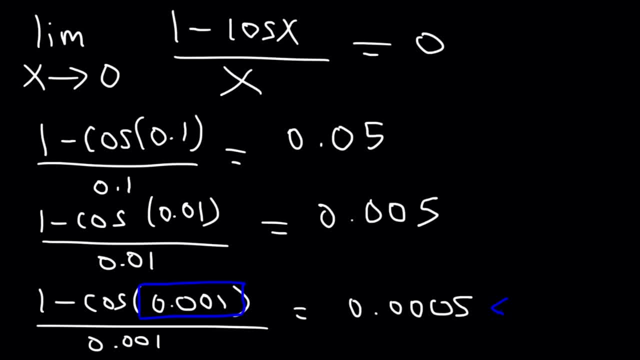 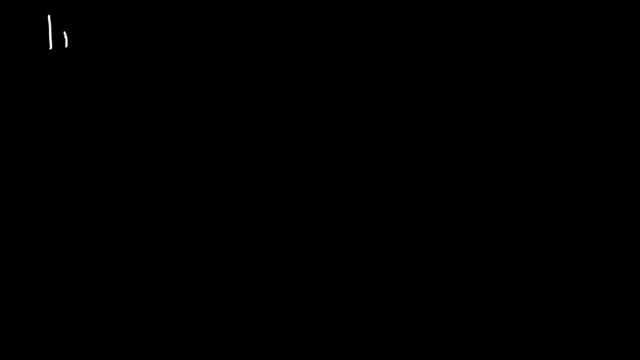 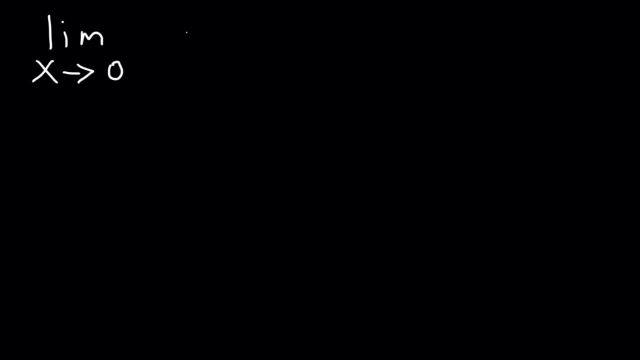 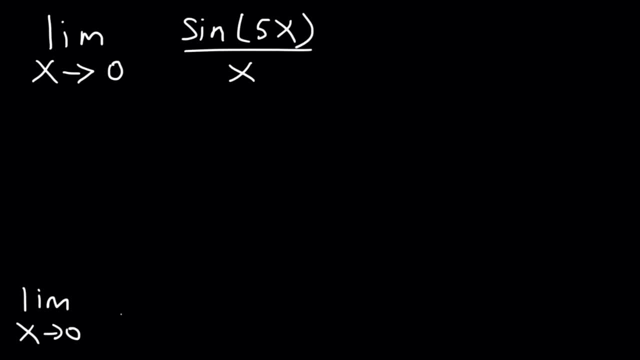 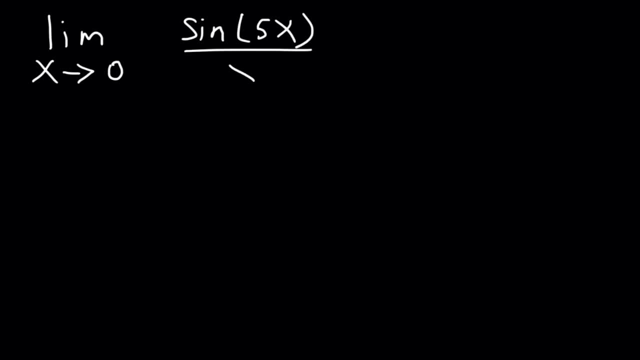 What is that equal to? Now, keep in mind: we know that the limit as x approaches 0, of sine x divided by x is 1.. For those of you who know how to solveержives, for those of you who quickly want to see the answer, it's going to be 5x divided by 1x. 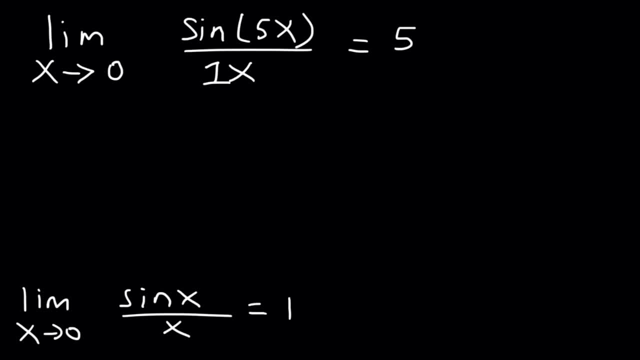 which is 5, but you got to show your work, though, but that's just a quick way to get the answer. for those of you who want that, what you need to do is multiply the top and the bottom by 5. and we're going to take this 5 and move it over here. 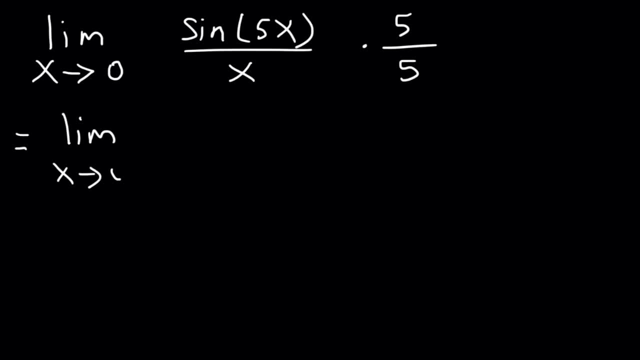 so this is equal to the limit as x approaches 0 sine 5x divided by 5x times 5.. now what we're going to do is we're going to use substitution. let's say that y is equal to 5x, so notice that the limit as x approaches 0 of 5x. 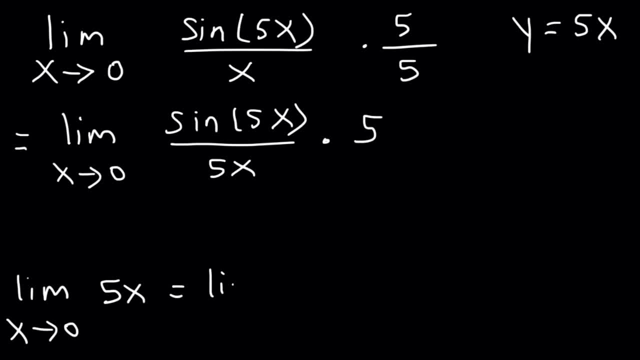 that's equal to 0. that's also equivalent to the limit, as y approaches 0, of y, since y is equal to 5x. as x approaches 0, we know that this limit becomes 0, and this is also equal to 0, so therefore they're equal to each other. 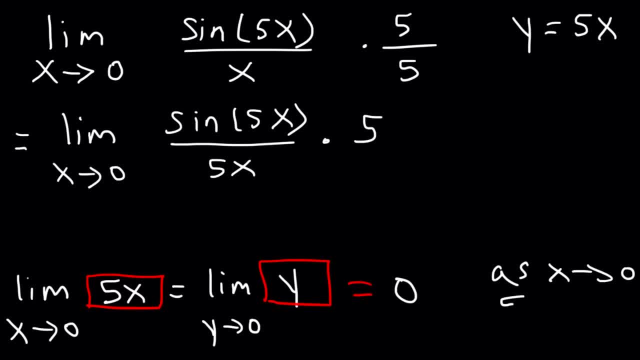 so, therefore, as x approaches 0, 5x becomes 0, and 5x is y, so y becomes 0 too. so by making that statement, we need to realize that we can now change the limit to this expression. we can say the limit as y approaches 0 sine y divided by y times 5.. so all we did is we substituted: 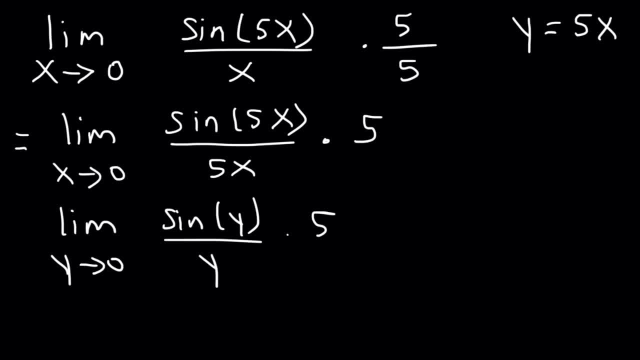 5x with y. now we can use the formula: if the limit as x approaches 0 is equal to 5x, then we're going to substitute 5x with y. so we're going to substitute 5x with y. now we can use the formula. if the limit as x approaches 0 is equal to 0. 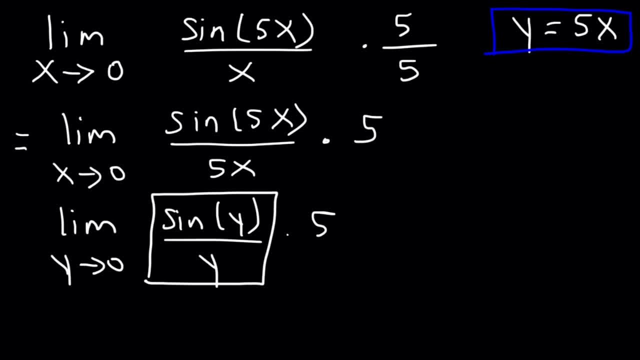 as x approaches 0 for sine x over x. if that's 1, then the limit as y approaches 0 of sine y divided by y must also be 1. so this is going to be 1 times 5, which is equal to 5, and that's the answer. 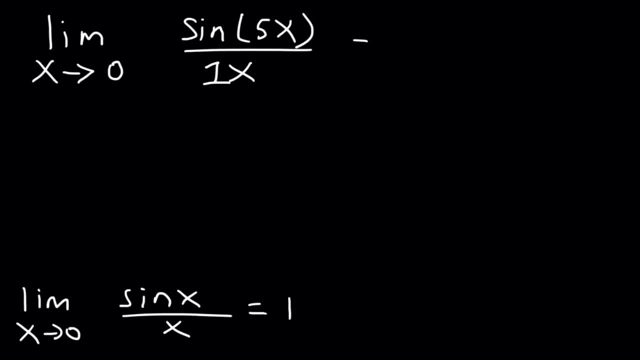 you got to show your work, though, but that's just a quick way to get the answer. for those of you who want that, what you need to do is multiply the top and the bottom by 5, and we're gonna take this 5 and move it over here, so this is: 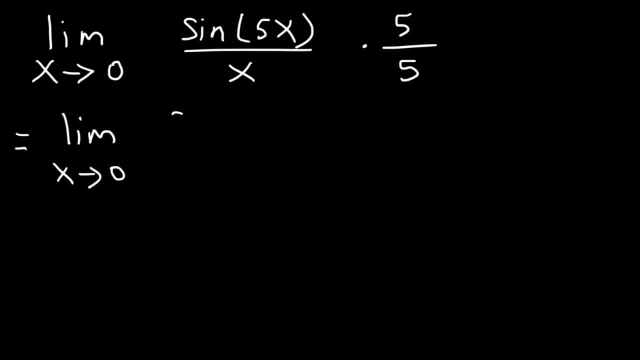 equal to the limit as X approaches 0 sine 5x divided by 5x times 5. now we're going to do is we're going to use substitution. let's say that Y is equal to 5x, so notice that the limit as X approaches 0 of 5x, that's equal to 0. 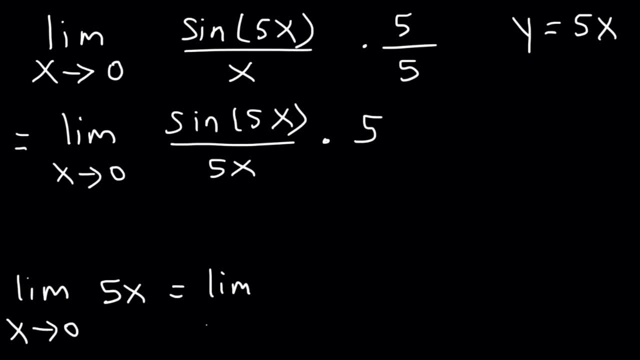 that's also equivalent to the limit of 5x as Y approaches 0 of Y. since Y is equal to 5x as X approaches 0, we know that this limit becomes 0, and this is also equal to 0, so therefore they're equal to. 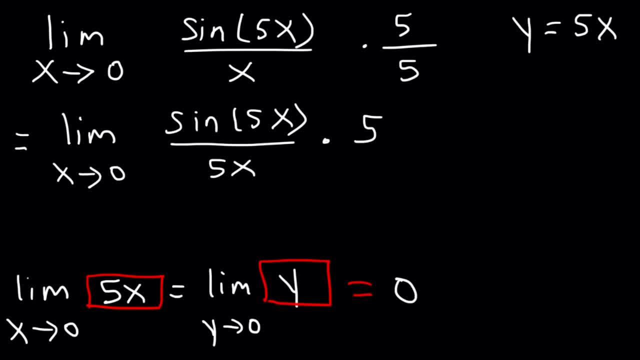 each other. so therefore, as X approaches 0, 5x becomes 0- you- and 5x is Y, so Y becomes 0 too. so I'm making that statement. we need to realize that we can now change the limit to this expression. we can say the limit as Y. 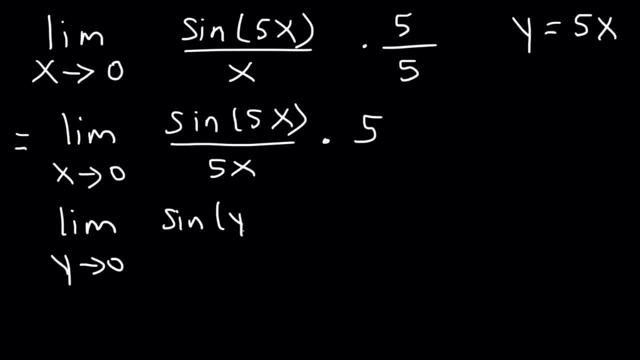 approaches 0 sine Y divided by Y times 5. so all we did is we substituted 5x with Y. now we can use the formula: if the limit as X approaches 0 for sine X over X, if that's 1, then the limit as Y approaches 0 of sine Y divided by Y must also be 1. 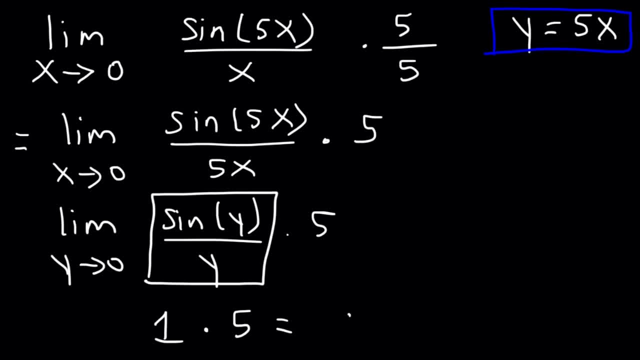 so this is going to be 1 times 5, which is equal to 5, and that's the answer. so what you want to do is you want to make these two values the same, and then you could replace it with a letter like Y and then evaluate the limit that way, and 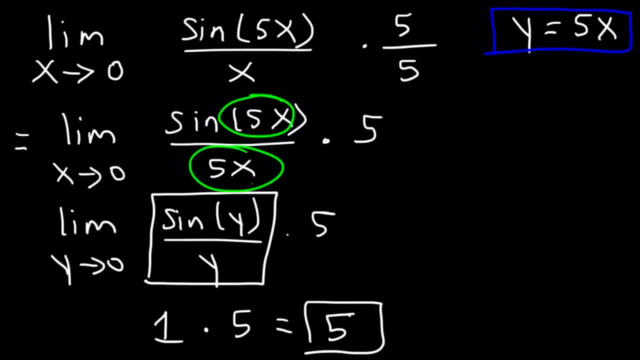 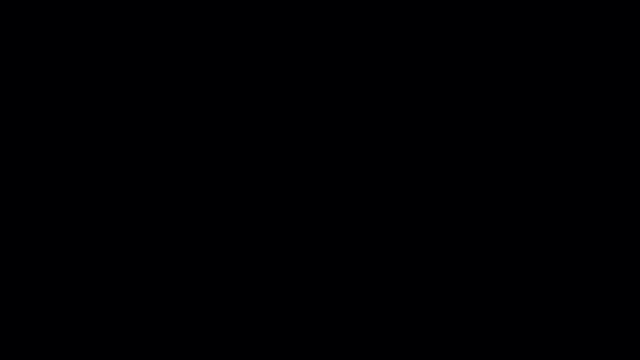 so what you want to do is you want to make these two values the same, and then you can replace it with a letter like y and then evaluate the limit. that way, let's try this problem: what is the limit as x approaches 0 of sine 2x divided by 5x? what do you think the answer to this problem is going to? 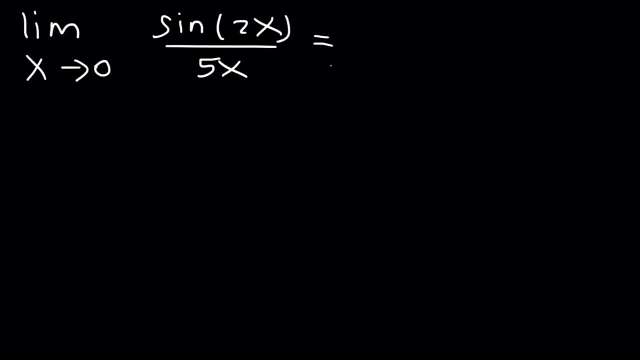 be. it turns out that it's just 2 divided by 5.. you can literally see it. but now let's show our work. so what we need to do is multiply the top and the bottom by 2 over 2.. what i'm going to do is switch. 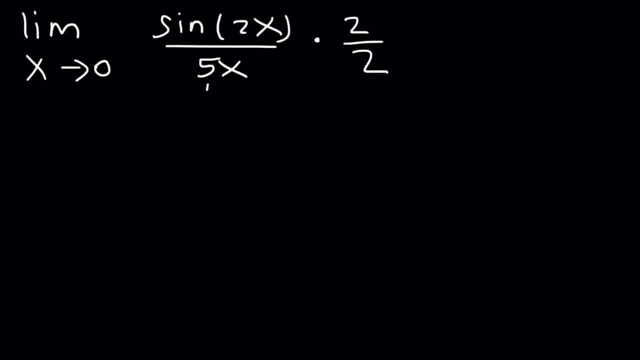 the 2 and the 5.. now this is going to give me 5 divided by 2, so i'm going to put these 2 together So we can rewrite it as the limit as x approaches 0, sine 2x divided by 2x times 2 over 5.. 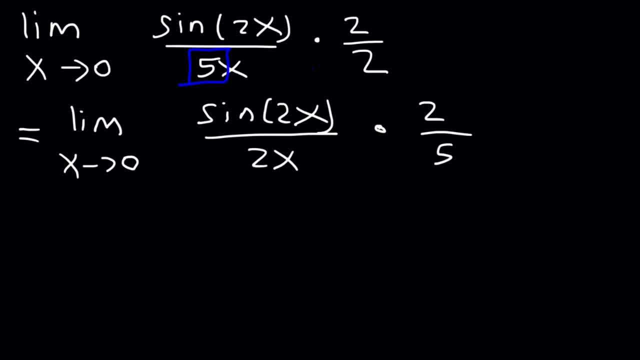 So I just switched the places of these two numbers: Five times two and two times five. they're both equal 10, so the value is still the same. Now, once these two values are the same, you can use substitution. So we're going to let y equal to 2x. 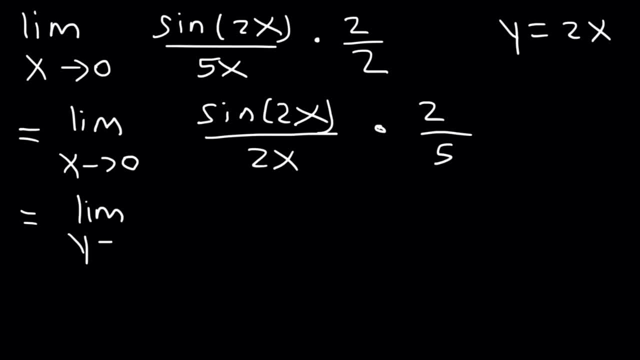 So therefore, we're going to change our expression as the limit as y approaches 0, sine y divided by y times 2 over 5.. Now we can use that one identity where the limit as x approaches 0, of sine x divided. 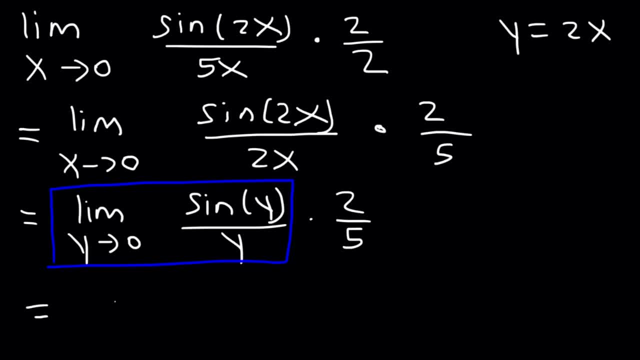 by x is 1.. So this expression in blue is also equal to 1.. So our final answer is 2 divided by 5, but now you can show your work. This is how you're going to show your work if you have to take it on a test. 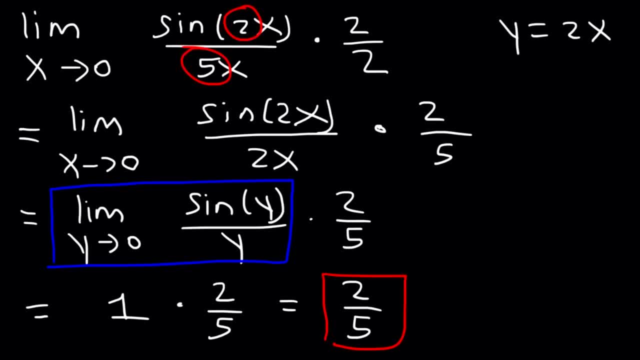 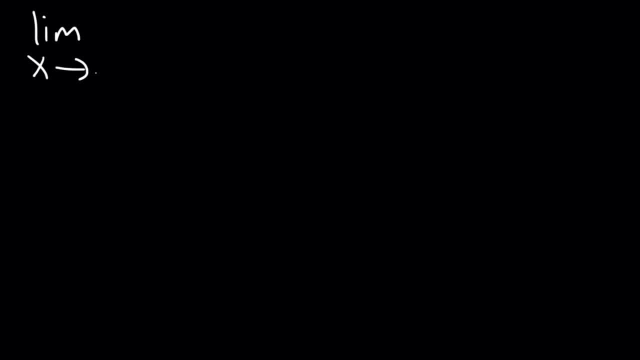 But if it's a multiple choice problem, you can clearly see that it's 2 over 5.. Now, what about this one? What is the limit as x approaches 0 for sine 7x divided by sine 3x? Feel free to pause the video. 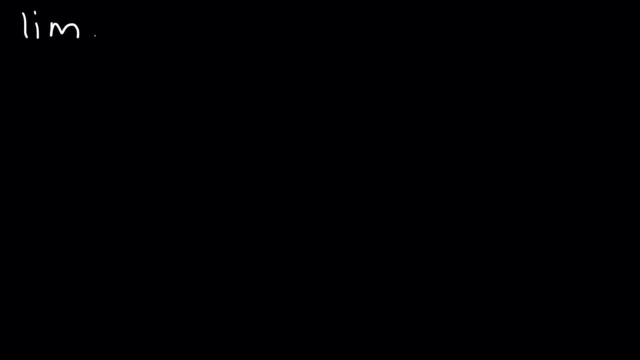 the end up to be the limit waiver. let's try this problem. what is the limit as X approaches 0, of sine 2x divided by 5x? what do you think the answer to this problem is going to be? it turns out that it's just 2 divided by 5. you can literally see it. now let's show our work. 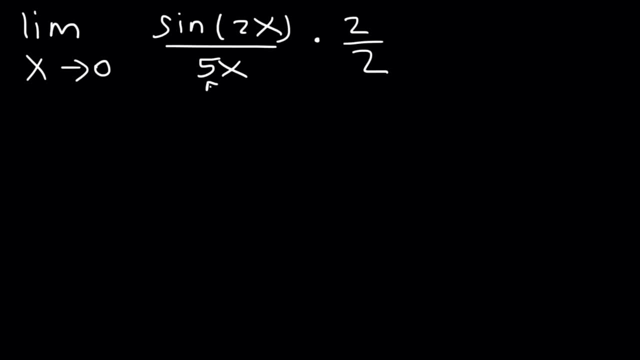 bottom by 2 over 2.. What I'm going to do is switch the 2 and the 5.. So we can rewrite it as the limit as x approaches 0, sine 2x divided by 2x times 2 over 5.. 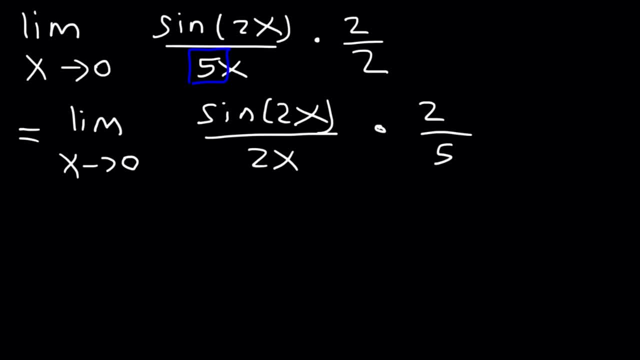 So I just switch the places of these two numbers: 5 times 2 and 2 times 5, they're both equal 10.. So the value is still the same. Now, once these two values are the same, you can use substitution. So we're going to let y equal to 2x. So therefore, 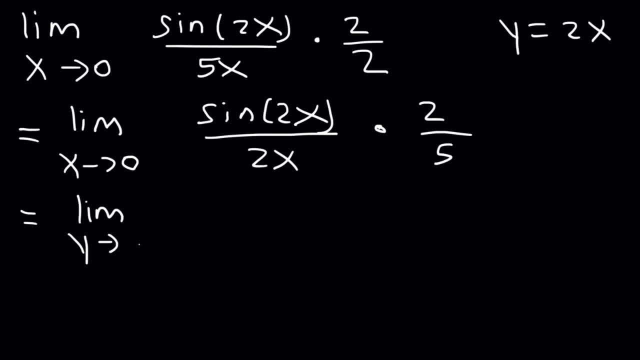 we're going to change our expression as the limit as y approaches 0, sine y divided by y times 2 over 5.. Now we can use that one identity where the limit as x approaches 0 of sine x divided by x is 1.. 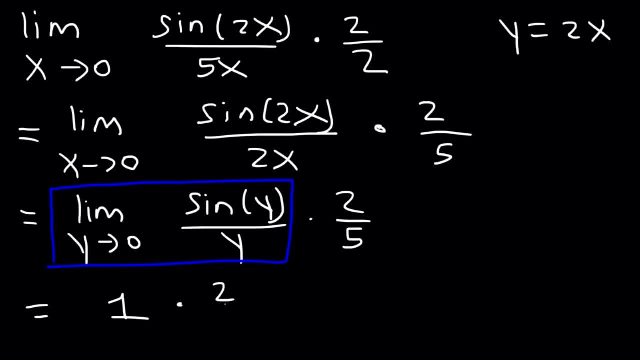 So this expression in blue is also equal to 1.. So our final answer is 2 divided by 5.. But now you can show your work. This is how you're going to show your work if you have to take it on a test, But if it's a multiple choice problem, you can clearly. 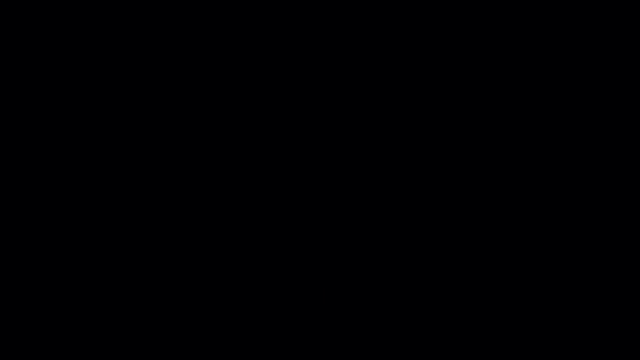 see that it's 2 over 5.. Now, what about this one? What is the limit as x approaches 0 for sine 7x divided by sine 3x? Feel free to pause the video and work on this problem. So just by looking at it, we. 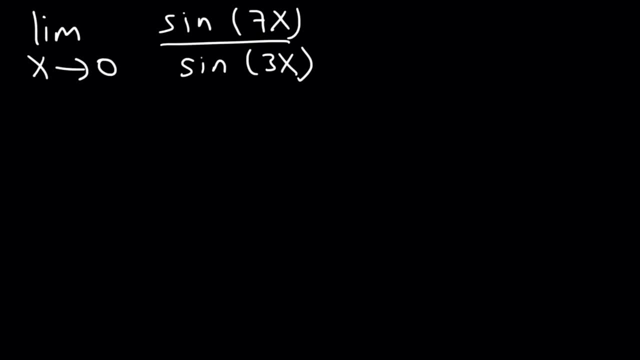 can see that it's 7 divided by 3.. But let's show our work. So what we're going to do is we're going to multiply the top and the bottom by 7 over 7,, 3 over 3, and x. 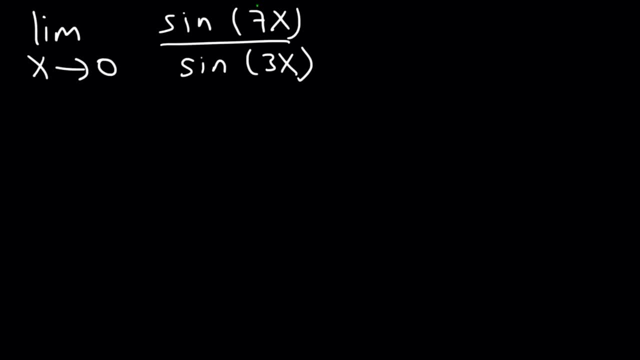 So just by looking at it, we can see that it's 7 divided by 3, but let's show our work. So what we're going to do is we're going to multiply the top and the bottom by 7 over 7,, 3 over 3, and x over x. 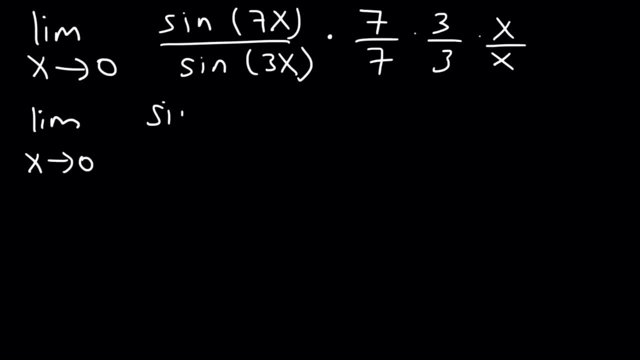 So now let's separate everything, So I'm going to leave the sine 7x on top. However, I need to put 7 and x. I need to move this over here. I want it to be below sine 7x. 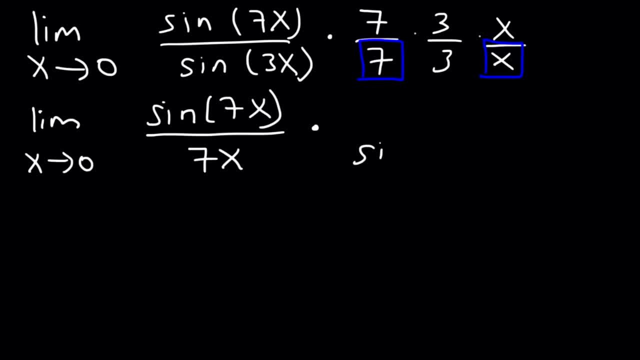 Now I need to do something with the sine 3x, So I have to keep it on the bottom, But on top I want 3x above it, So I'm going to write it here Now. what I have left over is 7 over 3, which I can put it in this third fraction. 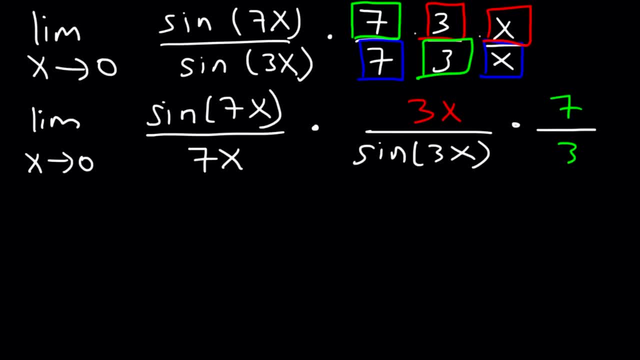 So I'm going to write it here. Now, what I have left over is 7 over 3, which I can put it in this third fraction, So I'm going to write it here. So every number has been accounted for. I just simply rearranged everything. 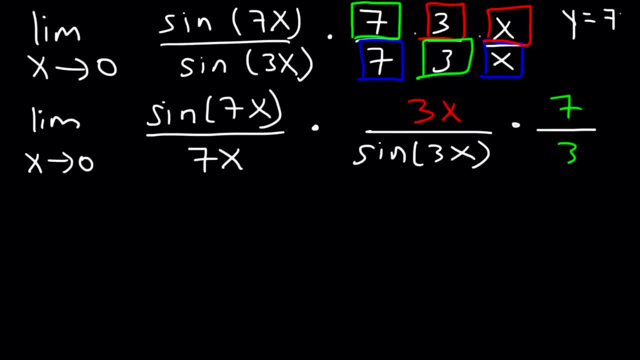 So let's say that y is equal to 7x, and let's say another variable, w, let's let it equal to 3x. So we're going to have the limit as y approaches zero sine y over y. So that's for this portion. 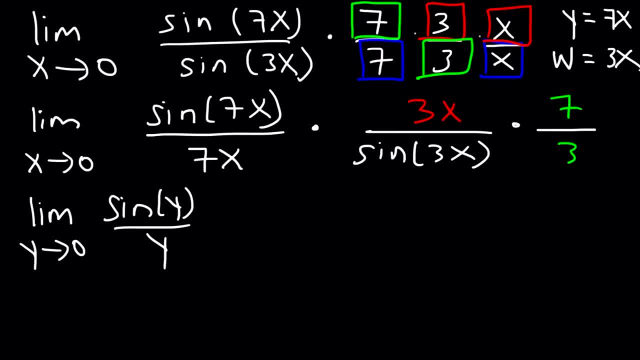 So that's for y, So that's for this portion, and then we're going to multiply that by the limit, as w approaches, 0 of w divided by sine w. since 3x, we set it equal to w, and then we're going to multiply. 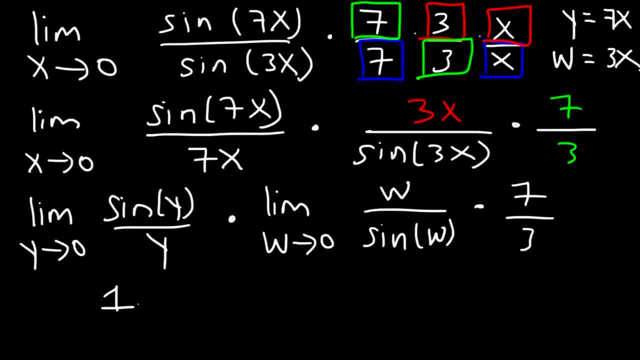 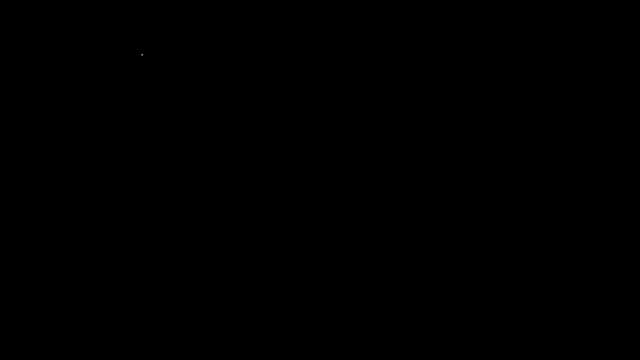 everything by 7 over 3.. So therefore this becomes 1,. this expression is also 1, and then times 7 divided by 3, so the final answer is 7 over 3.. And that's it. Let's try this one. The limit as x approaches 0,. tangent x divided by x. 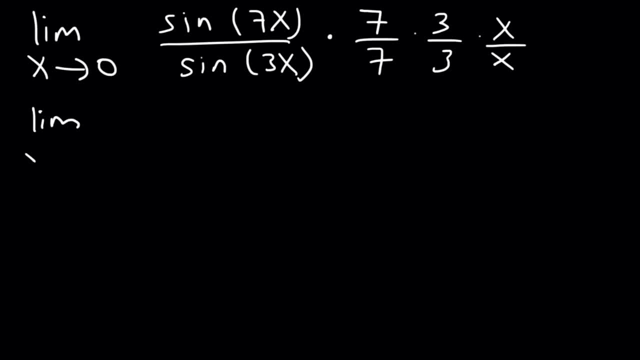 over x. So now let's separate everything. So I'm going to leave the sine 7x on top. However, I need to put 7 and x. I need to move this over here. I want it to be below sine 7x. Now I need to do something with the sine 3x, So I have to keep it on the bottom. 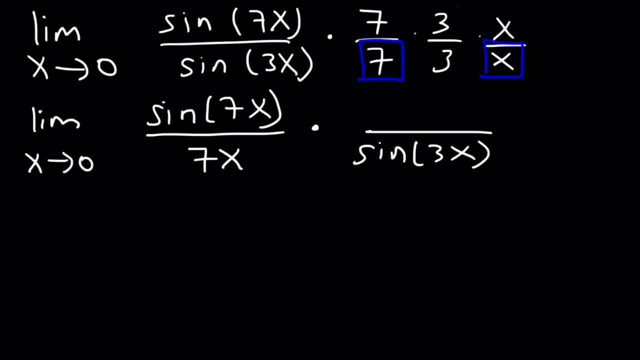 But on top I want 3x above it. So I'm going to write it here. Now, what I have left over is 7x over 7x. Now what I'm going to do is write everything down, So I'm going to write. 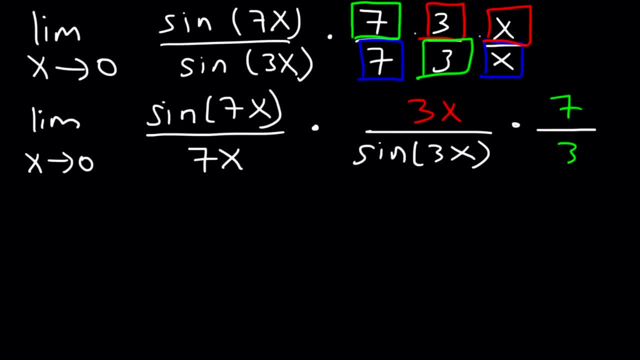 over 3, which I can put it in this third fraction. So every number has been accounted for. I just simply rearranged everything. So let's say that y is equal to 7x, and let's say another variable, w. let's let it equal to 3x. So we're going to have the limit as y approaches 0,. 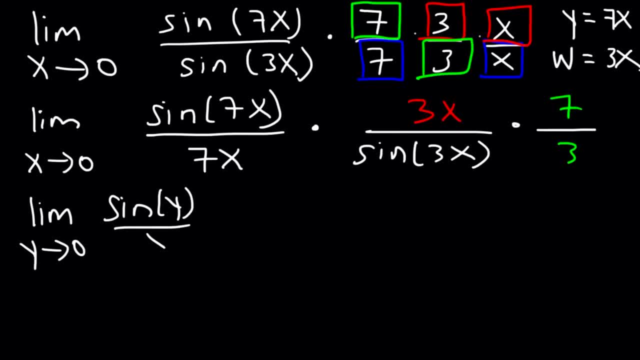 so sine y over y. So that's for this portion, And then we're going to multiply that by the limit, as w approaches 0, of w divided by sine w. since 3x, we set it equal to w, And then we're going to multiply. 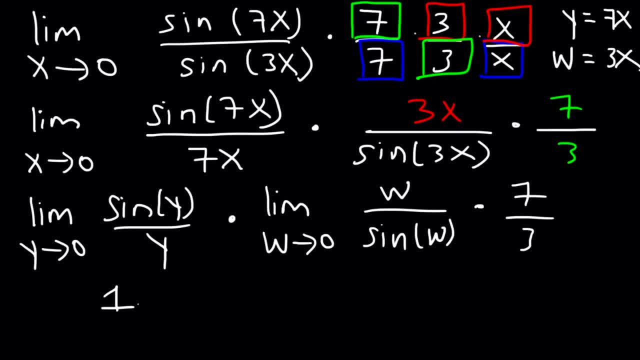 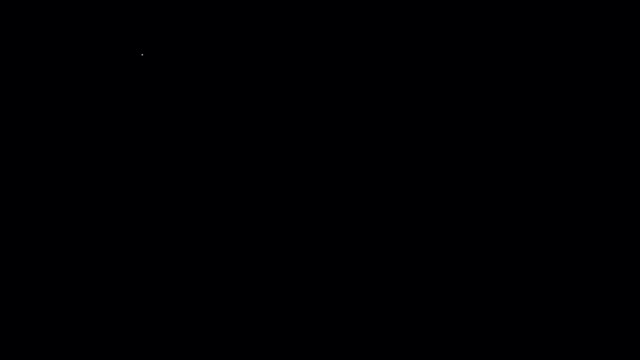 everything by 7 over 3.. So therefore this becomes 1.. This expression is also 1.. And then times 7 divided by 3.. So the final answer is 7 over 3.. And that's it. Let's try this one. The limit as x approaches 0, tangent x divided by x. 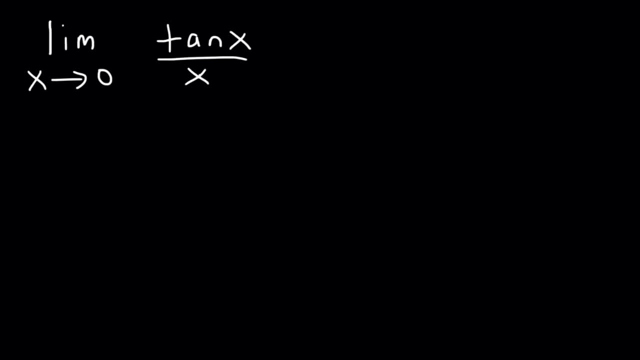 What do you think the answer to this problem is going to be? Well, tangent, we know, is 7. Sine divided by cosine. But first let's rewrite it like this: Let's separate x and tangent x, And now, in the next step, let's replace tangent. 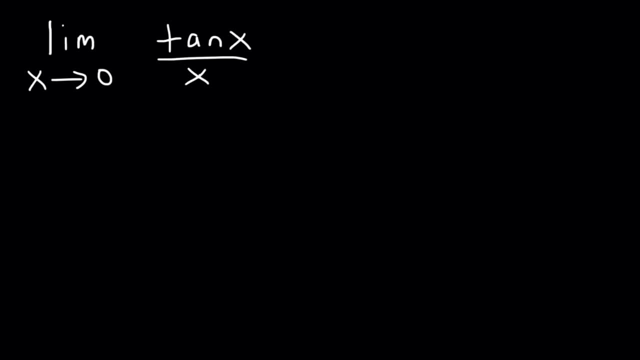 What do you think the answer to this problem is going to be? Well, tangent, we know, is sine divided by cosine. but first let's rewrite it like this: Let's separate x and tangent x, And now, in the next step, let's replace tangent with sine over cosine. 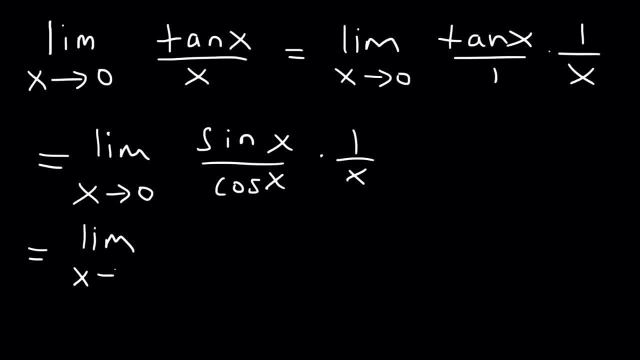 So this is equal to the limit as x approaches 0, sine x divided by x. I'm going to switch these two Multiplied by 1 over cosine x. Now, as we apply the limit sine x over x based on the formula will change to 1.. 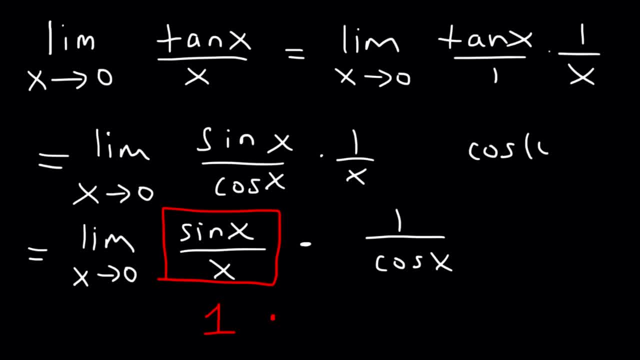 Now what about cosine? Cosine of 0 is 1, so as x approaches 0,, this becomes 1 as well. So the answer is 1.. And you can see it: Tangent x and sine x are very similar. 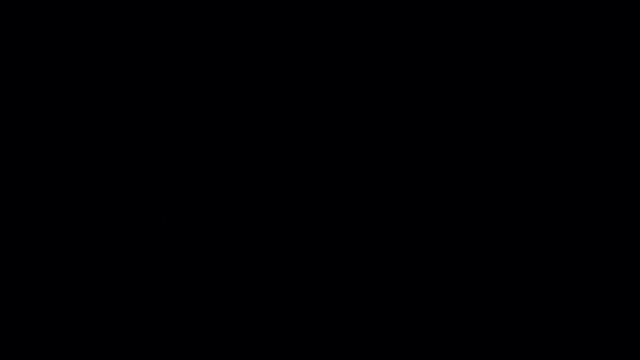 1x over 1x is 1.. Here's another example. Let's say if we want to find the limit as x approaches 0, of tan 4x divided by 3x, The answer is going to be 4 over 3, but let's prove it. 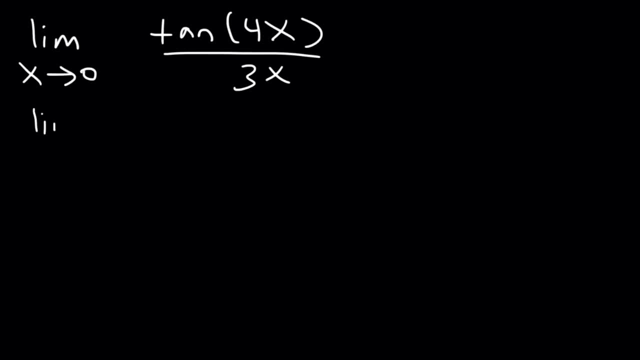 So first let's convert tangent into sine over cosine. So this is going to be sine 4x divided by cosine, 4x times 1 over 3x. Now we need to multiply the top and the bottom by 4x. 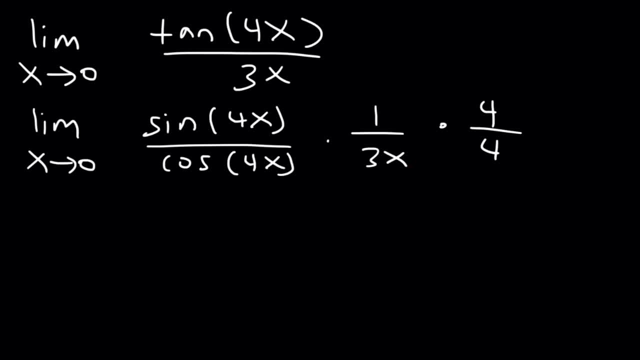 4 over 4.. So we need to take x and 4 and move it under sine. So this is equal to the limit as x approaches 0.. Sine 4x divided by 4x times 1 over cosine, 4x times 4 over 3.. 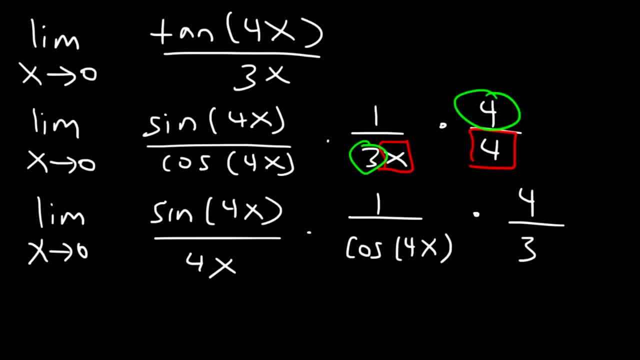 We had a 4 on top And a 3 on the bottom. Now let's say that y is equal to 4x, So this becomes the limit as y approaches 0.. Sine y divided by y times 1 over cosine y times 4 over 3.. 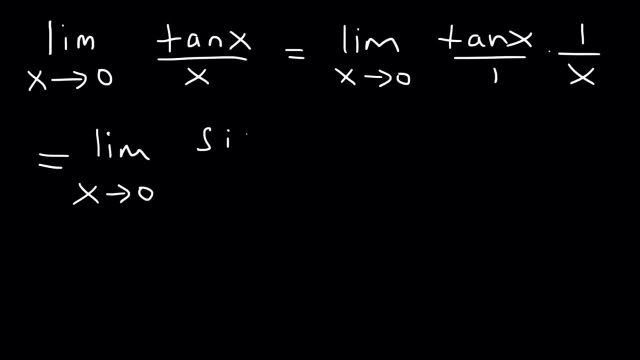 with sine over cosine. So this is equal to the limit as x approaches 0.. Sine x divided by x, Sine x divided by x: I'm going to switch these two multiplied by 1 over cosine x. Now, as we apply, the limit sine x over x, based on the formula, will change to 1.. 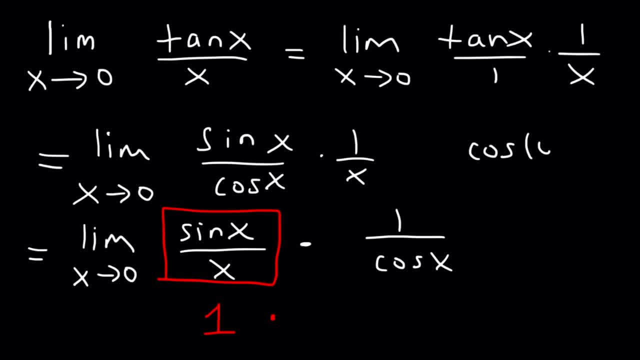 Now what about cosine? Cosine of 0 is 1, so as x approaches 0,, this becomes 1 as well. So the answer is 1.. And you can see it: Tangent x and sine x are very similar. 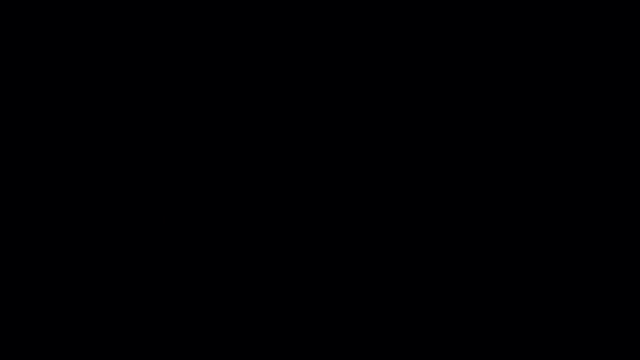 1x over 1x is 1.. Here's another example. Let's say if we want to find the limit, as x approaches 0, of tan 4x divided by 3x, The answer is going to be 4 over 3, but let's prove it. 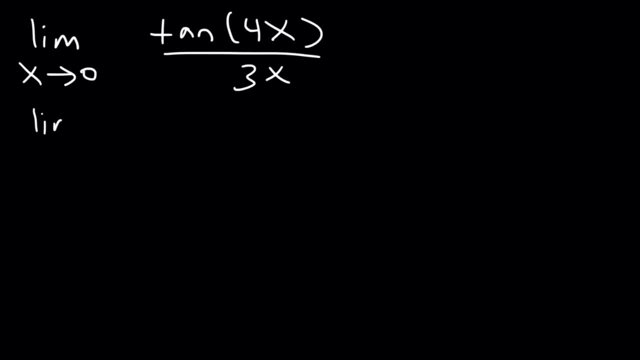 So first let's convert tangent into sine over cosine. So this is going to be sine 4x divided by cosine, 4x times 1 over 3x. Now we need to multiply the top and the bottom by 4 over 4.. 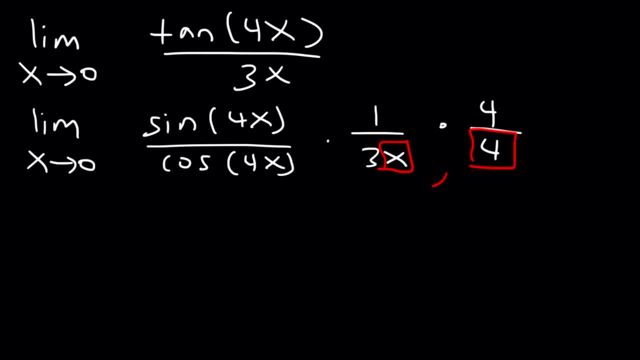 So we need to take x and 4 and move it under sine. So this is equal to the limit as x approaches 0.. Sine 4x divided by Sine 4x divided by 4x times 1 over cosine, 4x times 4 over 3.. 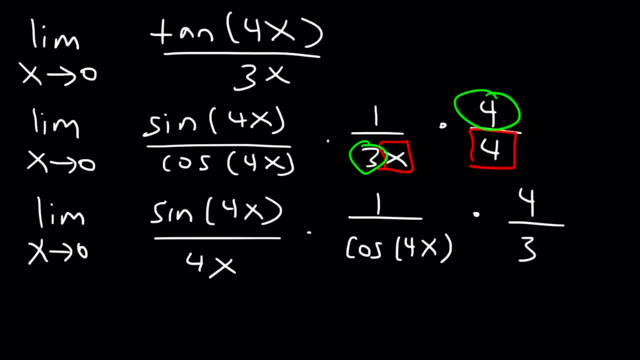 We had a 4 on top and a 3 on the bottom. Now let's say that y is equal to 4x, So this becomes the limit as y approaches 0.. Sine y divided by y times 1 over 4x. 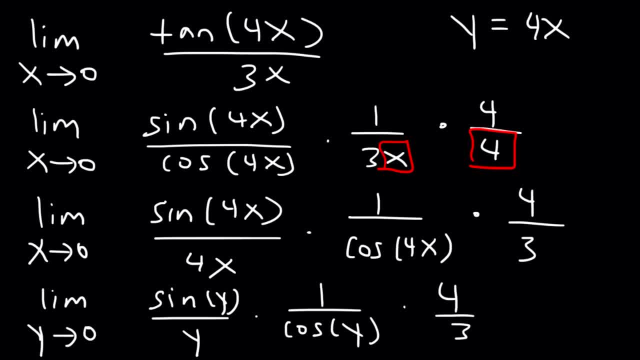 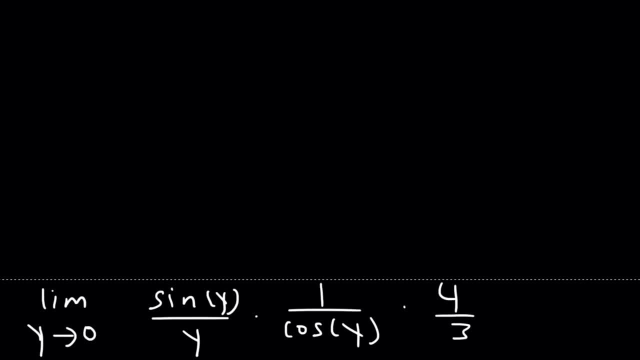 Or cosine y times 4 over 3. Sine y over y will change into 1.. Cosine 0 is 1.. So the final answer is going to be 4 over 3.. What about this one? The limit as x approaches. 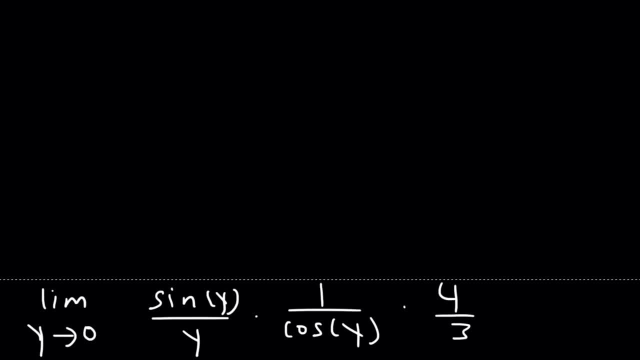 Sine y over y will change into 1.. So this becomes cosine 0.. So this actually becomes cosine 1 over 3.. And the final answer is going to be negative 6 times x. So the final answer is going to be 2 over 3,. 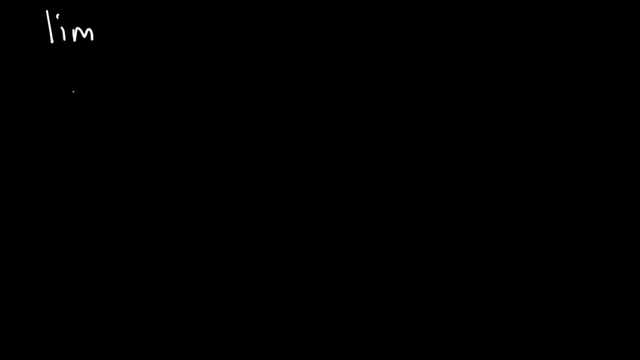 but we can't come back to that. Cosine 0 is 1, so the final answer is going to be 4 over 3.. What about this one? The limit, as x approaches 0, of 1 minus cosine x divided by x, that's equal to 0. 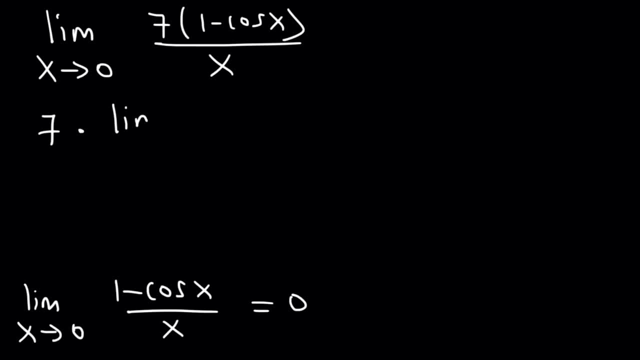 So, to show our work, we're going to separate 7 from everything else. So we know this portion here is 0.. So our answer is going to be 7 times 0, which is 0.. Now let's try a different example. 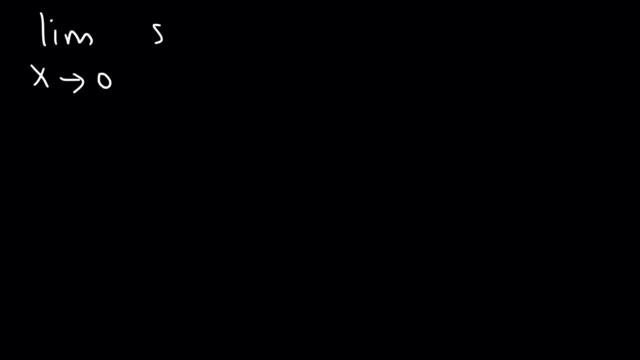 What is the limit as x approaches 0? Sine squared x divided by x. Take a minute and try that problem. So sine squared is basically sine x times sine x. So we have sine x over x times x. Now let's separate this into two limits. 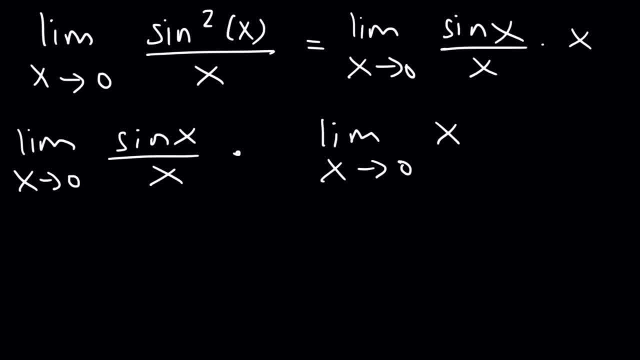 The limit as x approaches 0 of sine x divided by x, we know that's 1.. The limit as x approaches 0 of x: well, you can use direct substitution. that's going to be 0. So 1 times 0 is 0.. 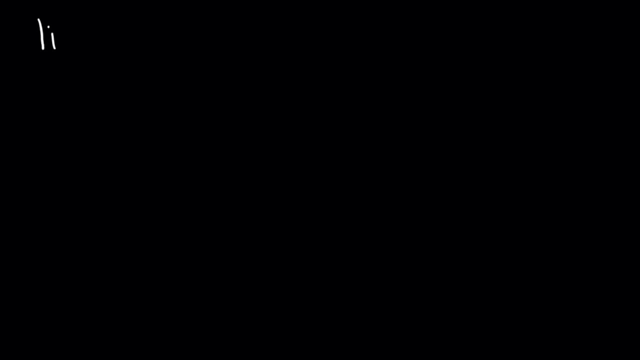 So this is the final answer. Consider this one: The limit as x approaches 0, sine of x squared divided by x. What's the answer? Well, what we need to do first is we need to multiply the top and bottom by x. 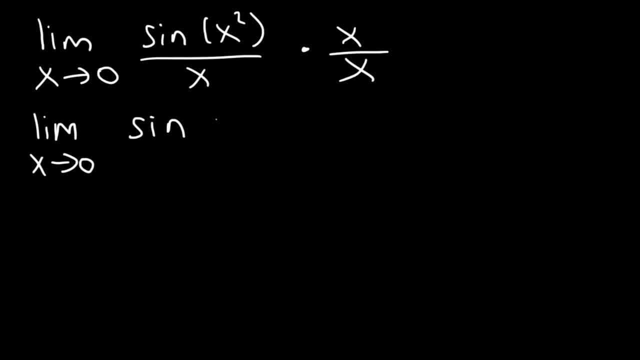 So we're going to get the limit as x approaches 0, sine of x squared divided by x squared. So we combine these two together And then we have an x on top left over. Now let's use substitution. Let's set y equal to x squared. 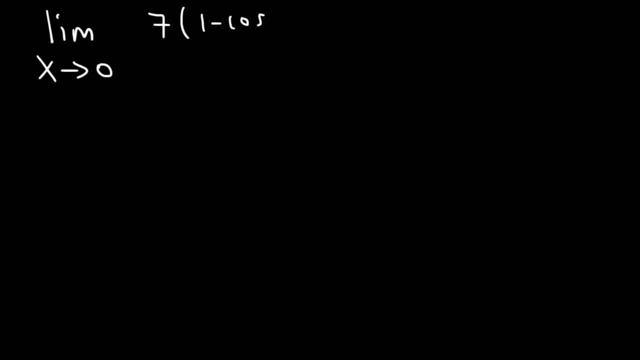 7 times 1 minus cosine x divided by x. What's the answer Now? if you recall the limit, as x approaches 0, of 1 minus cosine x divided by x, That's equal to 0.. So to show our work, we're going to separate 7 from everything else. 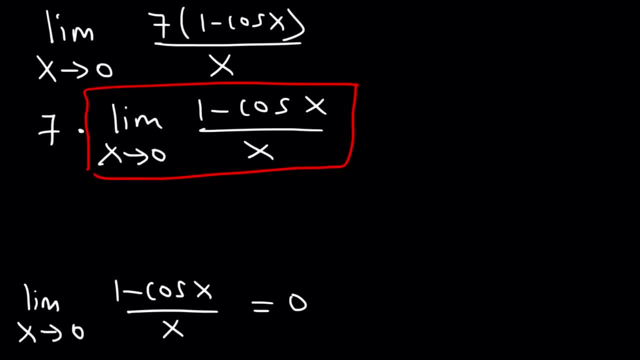 So we know this. So this portion here is 0.. So our answer is going to be 7 times 0, which is 0.. Now let's try a different example. What is the limit as x approaches 0?? Sine squared x divided by x. 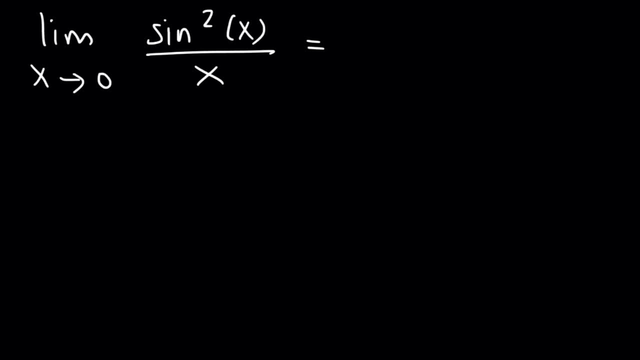 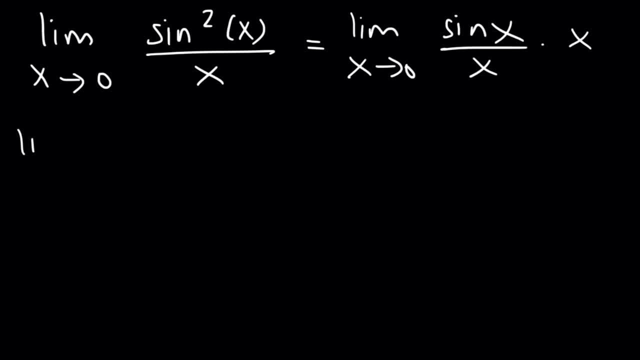 Sine x over x times x. Now let's separate this into two limits. The limit as x approaches 0 of sine x divided by x. we know that's 1. The limit as x approaches 0 of x. well, you can use direct substitution. 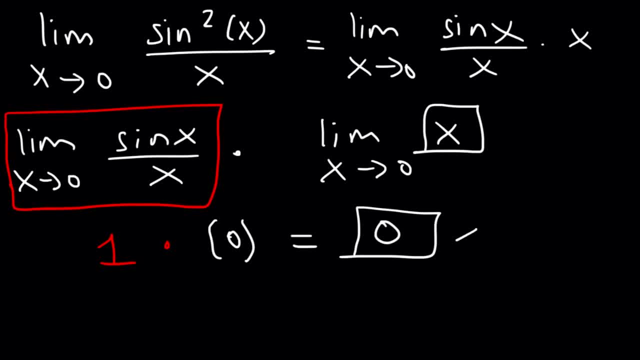 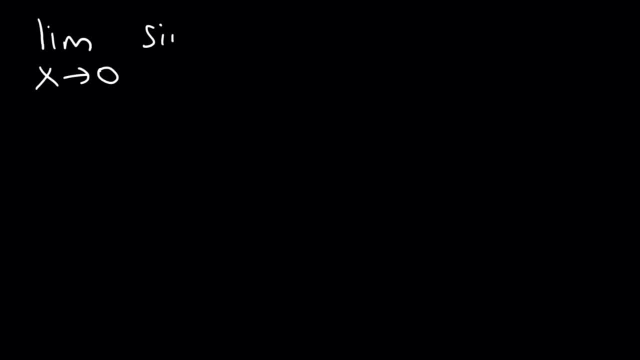 That's going to be 0.. So 1 times 0 is 0. So this is the final answer. Consider this one: The limit as x approaches 0: sine of x squared divided by x. What's the answer? Well, what we need to do first is we need to multiply the top and bottom by x. 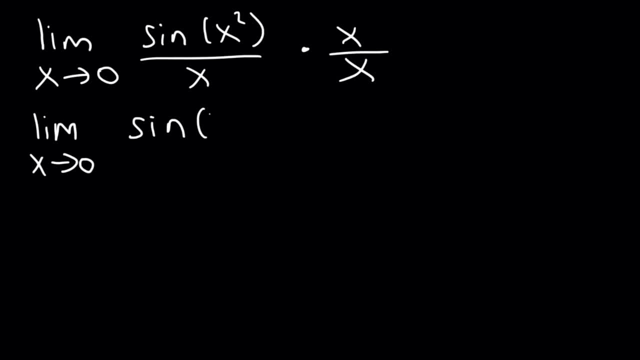 So we're going to get the limit as x approaches 0, sine of x squared divided by x squared. So we combine these two together And then we have an x on top left over. Now let's use substitution. Let's set y equal to x squared.